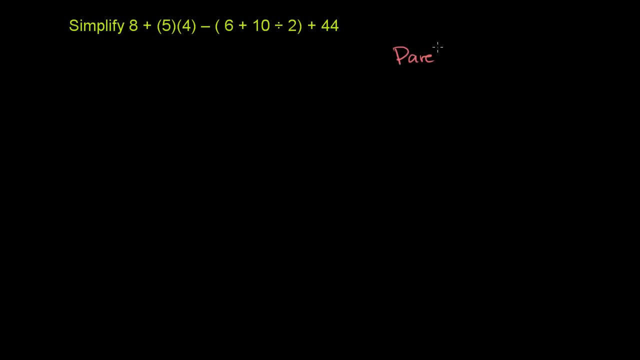 priority goes to parentheses, And those are these little brackets over here, or however you want to call them. Those are the parentheses right there. That gets top priority. Then after that, you want to worry about exponents. There are no exponents in this expression, but I'll just 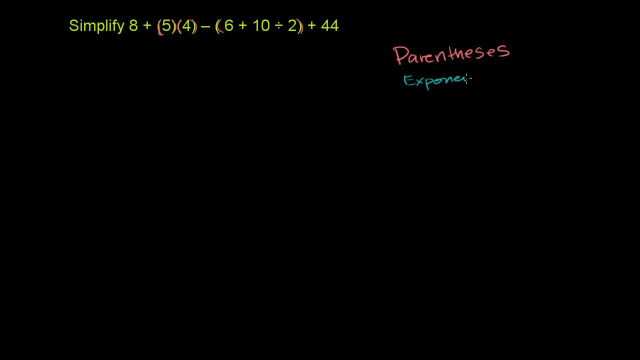 write it down, just for future reference. Exponents: One way I like to think about it is parentheses. that always takes top priority, But then after that we go in descending order, Or I guess we should say in descending order of how fast. 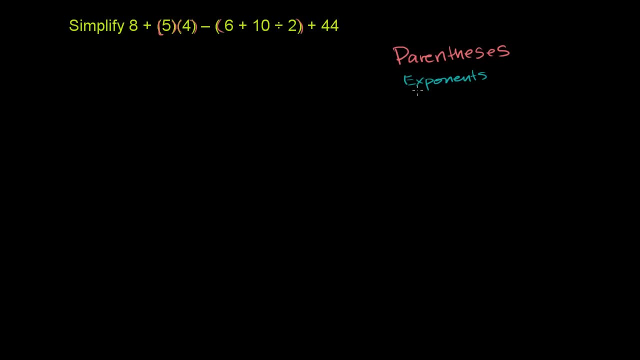 that computation is. And when I say fast how fast it grows, When I take something to an exponent, when I'm taking something to a power, it grows really fast. Then it grows a little bit slower or shrinks a little bit slower if I multiply or divide. 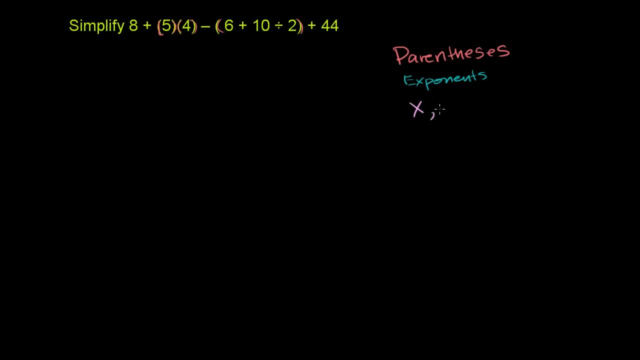 So that comes next. Multiply, or divide. Multiplication and division comes next, And then, last of all, comes addition and subtraction. So these are kind of the slowest operations. This is a little bit faster, This is the fastest operation. And then the parentheses, just no matter what. 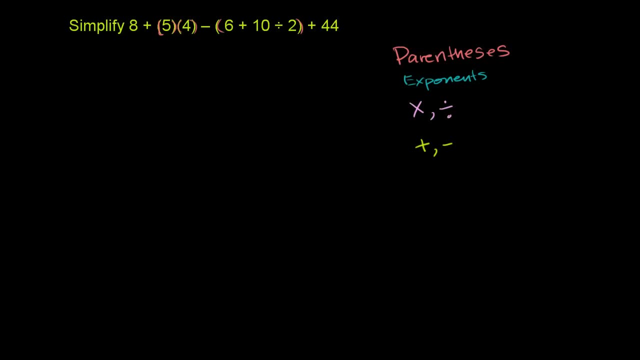 always take priority, So let's apply it over here. Let me rewrite this whole expression So it's 8 plus 5 times 4, minus in parentheses, 6 plus 10 divided by 2 plus 44.. So we're going to want to do the parentheses first. 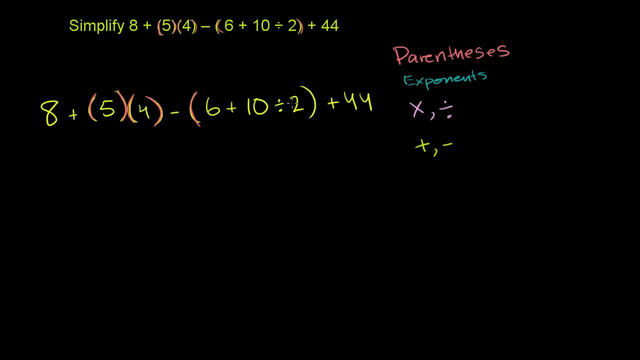 We have parentheses there And there. Now this parentheses is pretty straightforward. Well, inside the parentheses it's already evaluated, So we could really just view this as 5 times 4.. So let's just evaluate that right from the get-go. 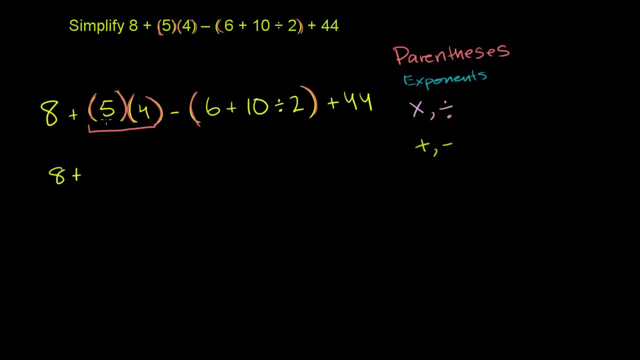 So this is going to result in 8 plus. and really, when you're evaluating the parentheses, if you evaluate this parentheses, you literally just get 5.. And then you evaluate that parentheses, you literally just get 4.. And then they're next to each other, so you multiply them. 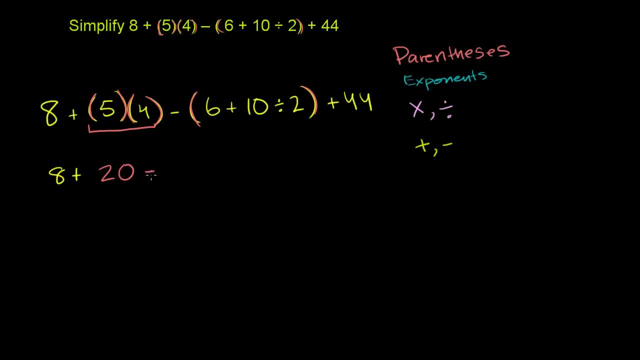 So 5 times 4 is 20.. Minus- Let me stay consistent. Let me stay consistent. Let me stay consistent with the colors: Minus. Now let me write the next parentheses right there And then inside of it. we need to evaluate this first. 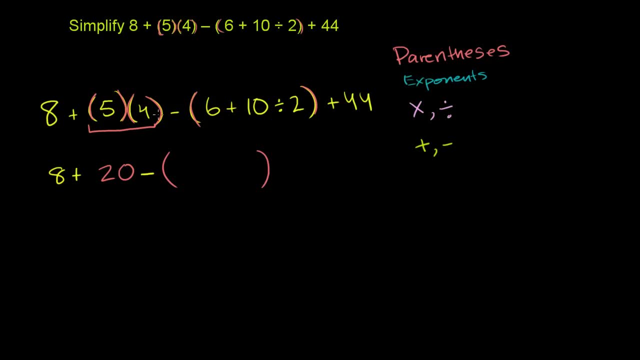 So let me close the parentheses right there, And then we have plus 44. So what does this thing right here evaluate? to this thing inside the parentheses? Well, you might be tempted to say, well, let me just go left to right.